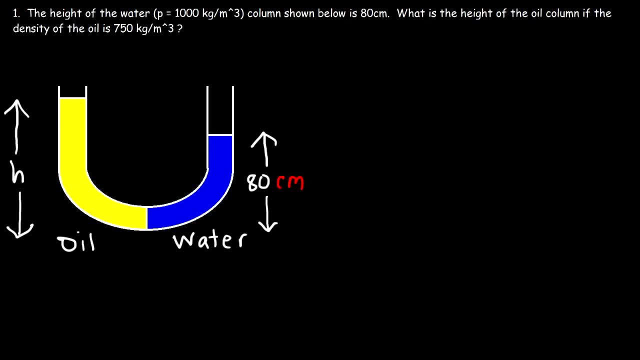 In this problem. we have a U-shaped tube and we're given the height of the water. on the right side It's 80 centimeters and we have the density of the water as well. What is the height of the oil column if the density of the oil is 750 kilograms per cubic meter? 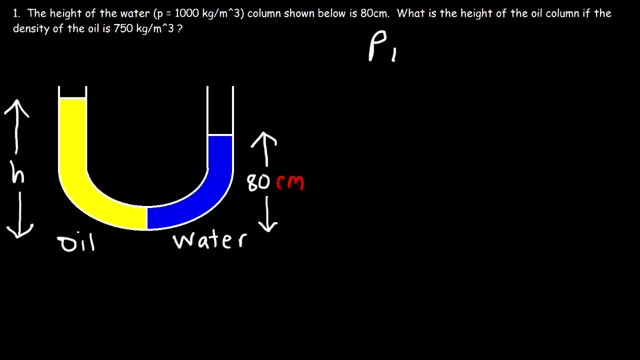 So, as I've mentioned before on other problems, the downward pressure on the left side has to equal the total downward pressure on the right side in order for the system to remain at equilibrium. So on the left side the tube is open to the air. 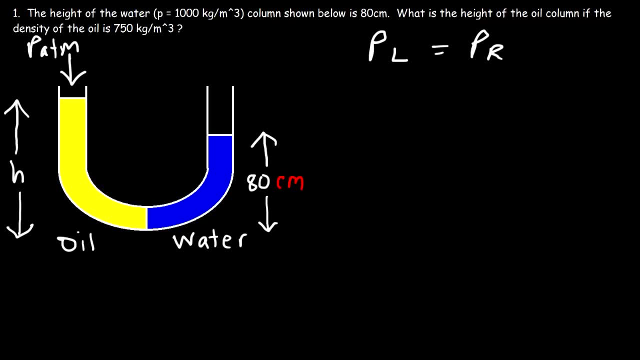 So we have the pressure of the atmosphere pushing down on the left side And we also have the weight of the oil pushing down on the left side. On the right side it's open to the air, so we have the atmospheric pressure on that side as well. 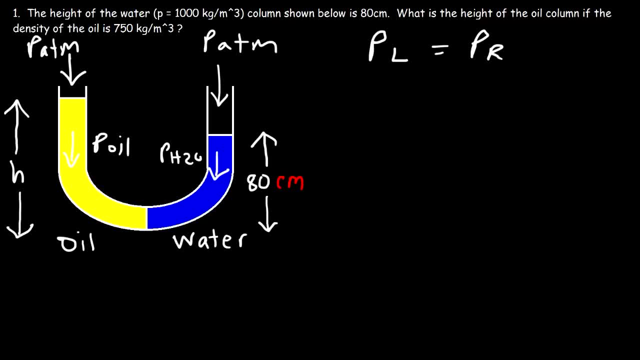 And then we have the pressure of the water on the right side. So on the left side we have the atmospheric pressure and the pressure of the oil, And on the right side we have the pressure of the water and the pressure of the atmosphere. 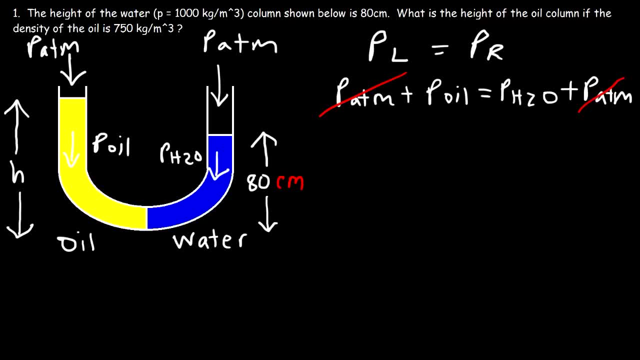 So these two will be the same. We don't have to worry about that. So, therefore, the downward pressure due to the weight of the oil is equal to the downward pressure due to the weight of the water And the pressure due to the weight of any fluid. 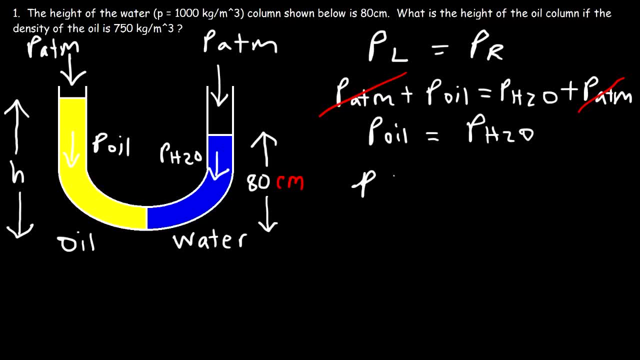 is equal to the density of that fluid times the gravitational acceleration, times the height, And so I'm going to call this P2gh2.. Now, g is the same, So this is the formula that we need for this type of problem: The density of the oil times the height of the oil. 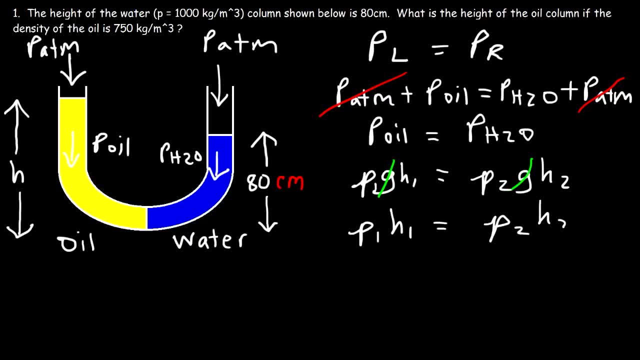 is equal to the density of the water, times the height of the water. So the density of the oil is 750.. We're looking for the height of the oil column. The density of water is 1,000. And the height of the water column is 80 centimeters. 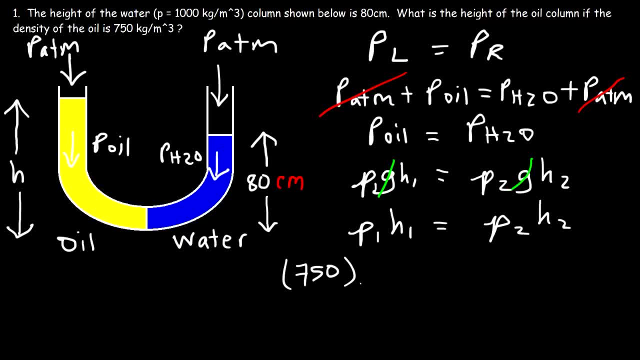 So the density of the oil is 750.. We're looking for the height of the oil column. The density of water is 1,000.. And the height of the water column is 80 centimeters. So it's going to be 1,000 times 80 divided by 750. 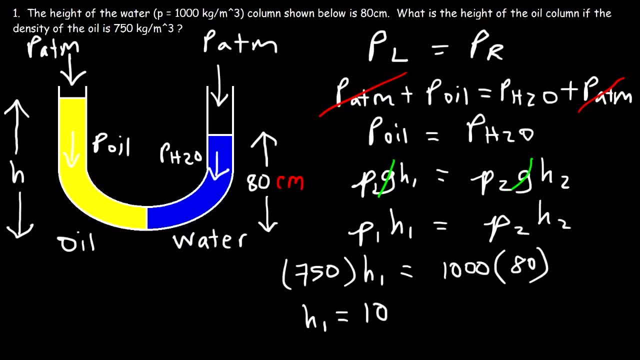 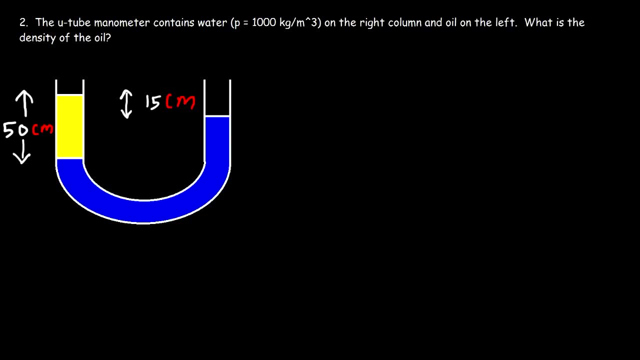 So the height of the oil column is 106.7 centimeters, And so this is the answer Number two. The U-tube manometer contains water on the right column and oil on the left. What is the density of the oil? 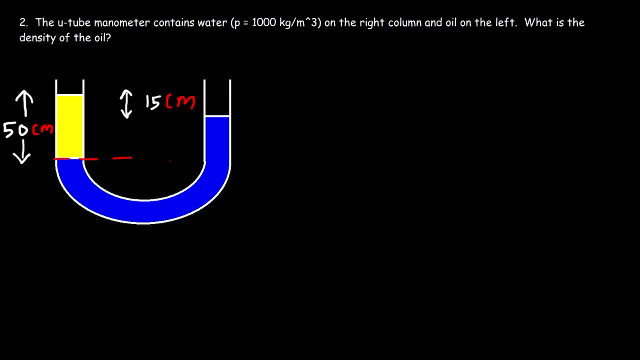 So let's create a reference level. Let's say this is the reference level. So that means the height of water above the reference level has to be the difference between 50 and 15.. So therefore, that's 35 centimeters Now, because 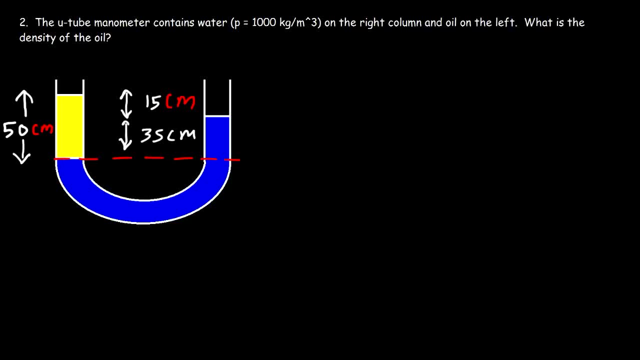 this fluid is the same on the bottom, we don't have to worry about it. The only part that's different is the height of the oil above the reference level and the height of the water above the reference level. It's all the same here, so we don't have to worry about that. 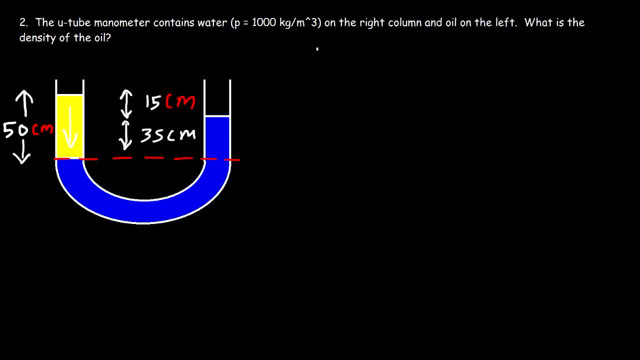 So we could say that the pressure due to the oil on the left has to be equal to the pressure due to the water above the reference level on the right. In order to do that- we're going to have to do this In order for this system to be at equilibrium. 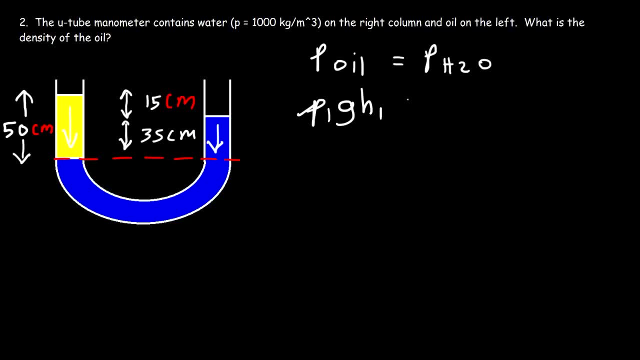 So rho 1 times g times h1 has to equal rho 2 times g times h2.. And, as always, we could cancel g, So we're going to come up with this equation again. So the density of the oil is what we're looking for in this problem. 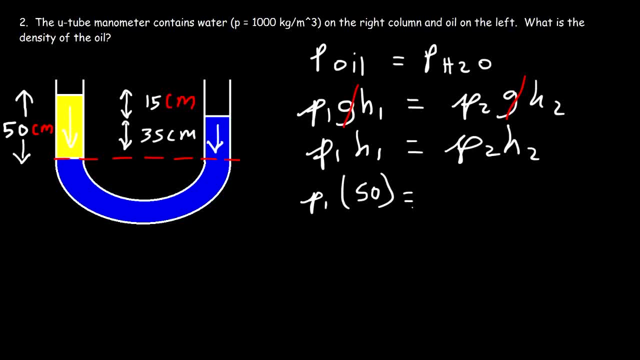 The height of the oil is 50 centimeters, The density of water is 1000. And the height of water above the reference level is 35 centimeters. Now make sure the units are the same. If they're not, you need to adjust it. 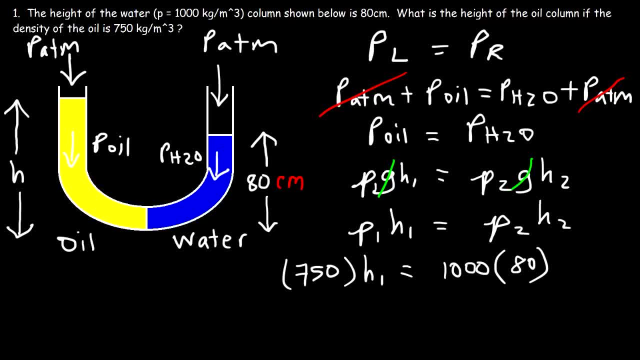 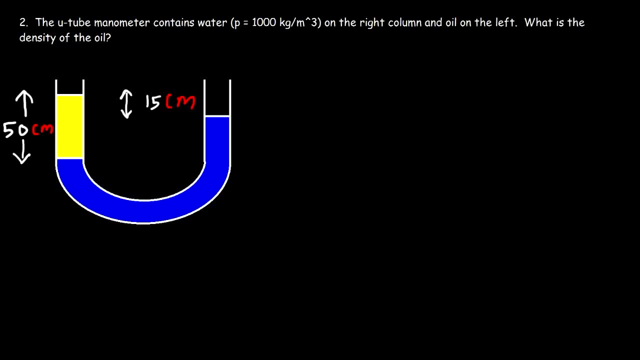 So it's going to be 1,000 times 80, divided by 750.. So the height of the oil column is 106.7 centimeters, And so this is the answer Number two. The U-tube manometer contains water. 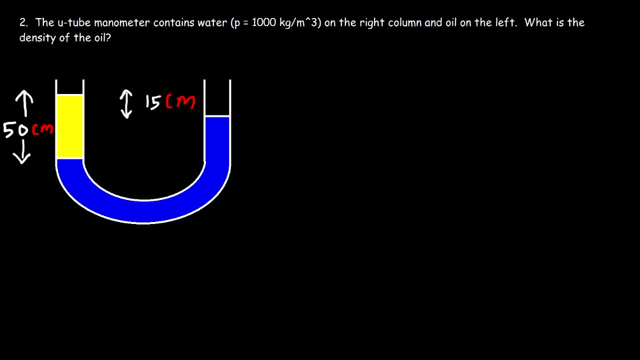 on the right column and oil on the left. What is the density of the oil? So let's create a reference level. Let's say this is the reference level. So that means the height of water above the reference level has to be the difference between 50 and 15.. 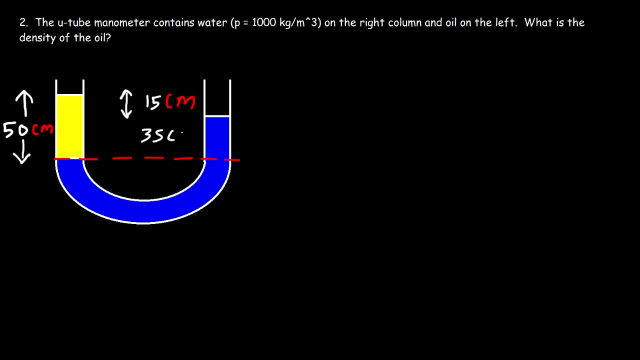 So therefore, that's 35 centimeters Now. because this fluid is the same on the bottom, we don't have to worry about it. The only part that's different is the height of the oil above the reference level and the height of the water above the reference level. 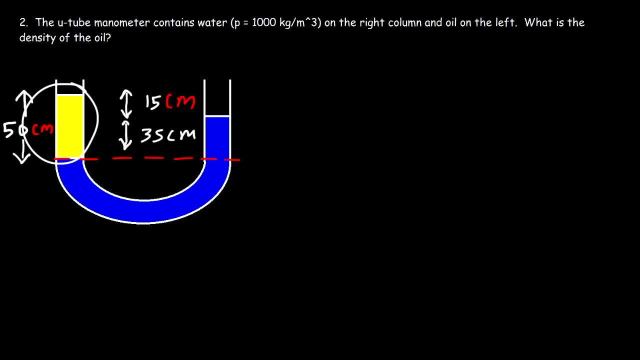 It's all the same here, so we don't have to worry about that. So we could say that the pressure due to the oil on the left has to be equal to the pressure due to the water above the reference level on the right In order for this system to be at equilibrium. 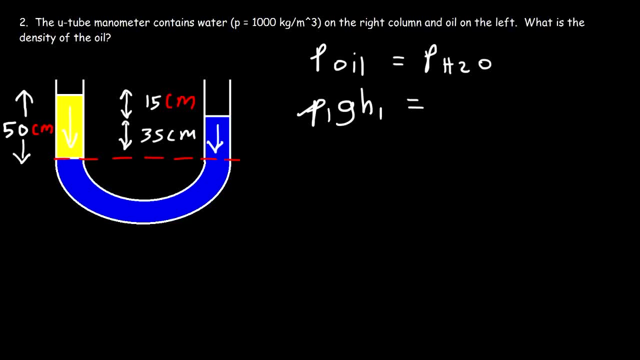 So Rho 1 times G times H1 has to equal Rho 2 times G times H2.. And, as always, we could cancel G, So we're going to come up with this equation again. So the density of the oil. 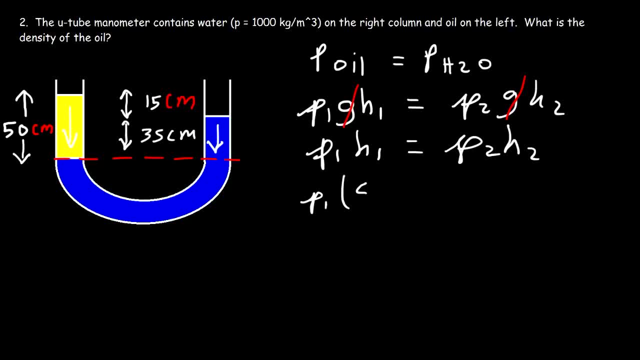 is what we're looking for in this problem. The height of the oil is 50 centimeters, The density of water is 1000. And the height of water above the reference level is 35 centimeters. Now make sure the units are the same. 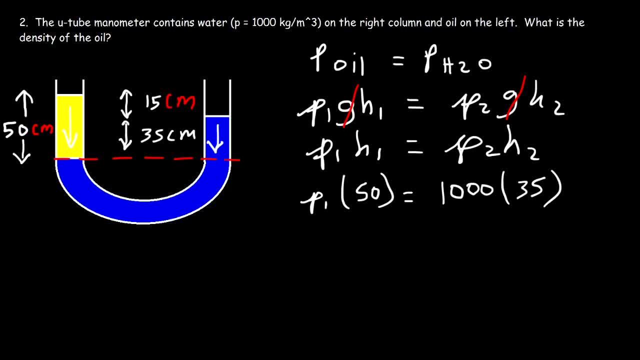 If they're not, you need to adjust it. So it's going to be 1000 times 35 divided by 50. So the density of the oil is 700 kilograms per cubic meter, And so that's the answer in this problem. 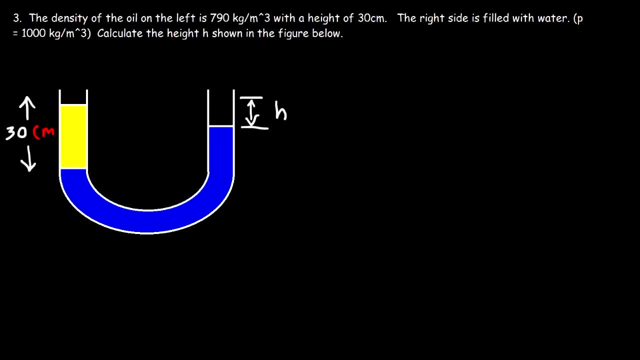 Number 3.. The density of the oil on the left is 790 kilograms per cubic meter. with a height of 30 centimeters, The right side is filled with water. Calculate the height H shown in the figure below. So we want to find this value. 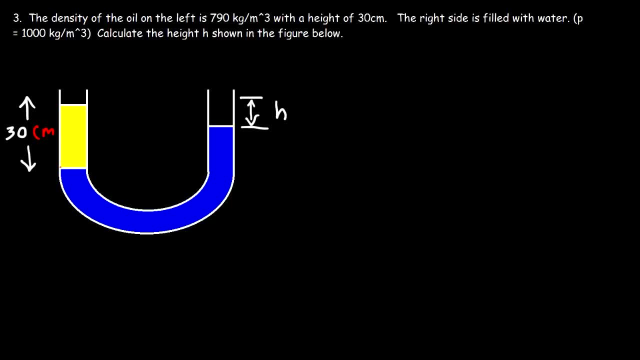 So go ahead and try this problem. Now let's establish a reference level, So let's call this height H1. Or rather H2.. That's going to be the height of the water above the reference level. So, just like before, we know the pressure. 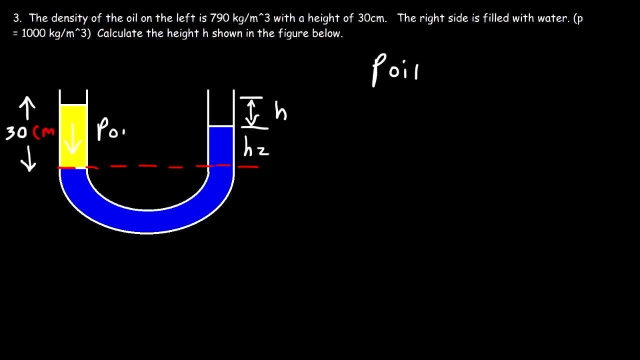 of the oil exerted on the left side has to equal the pressure of the water exerted on the right side, the portion that's above the reference level, And so that's going to be density times gravity times height. The density of the oil is 790.. 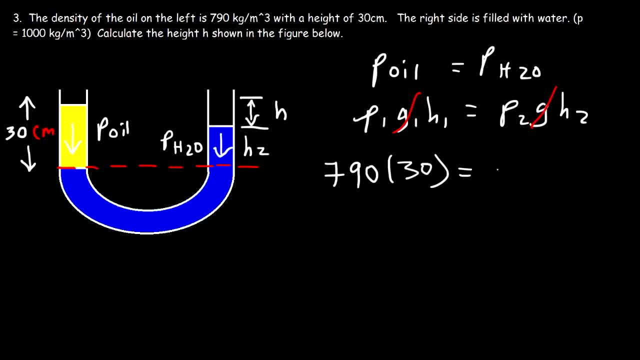 And the height of the oil is 30.. The density of water is 1000.. So let's calculate H2.. So it's 790 times 30 divided by 1000.. So H2 is 23.7 centimeters. 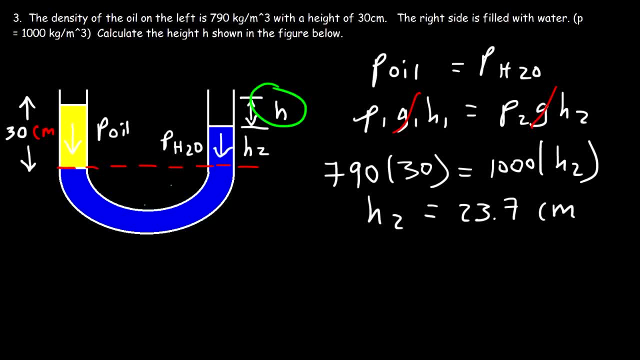 Now we're looking for this H, which is the difference between 30 and H2.. So H is 30 centimeters minus 23.7 centimeters, And so the answer is H2.. And so the answer is 6.3 centimeters. 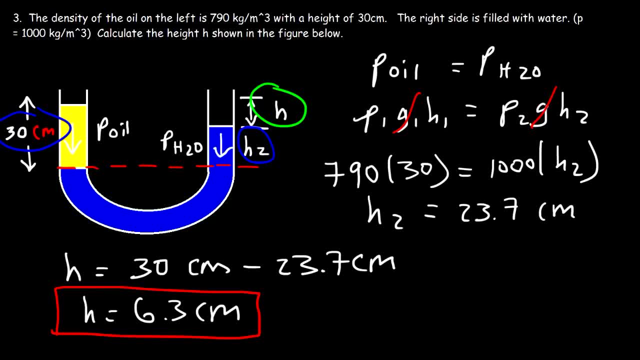 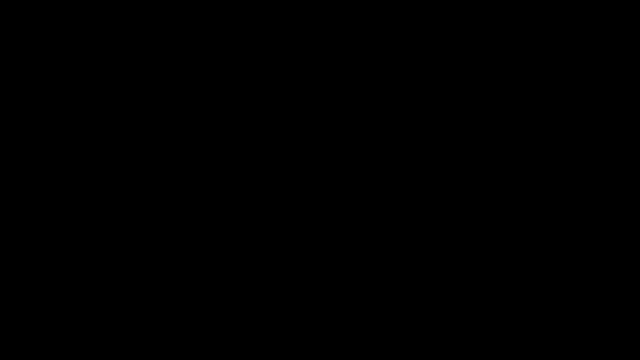 So the surface of the oil is 6.3 centimeters higher than the surface of the water. Well, of course, H2 would not be equal scale. It's just 19 centimeters cabover. Now if we look at H2, 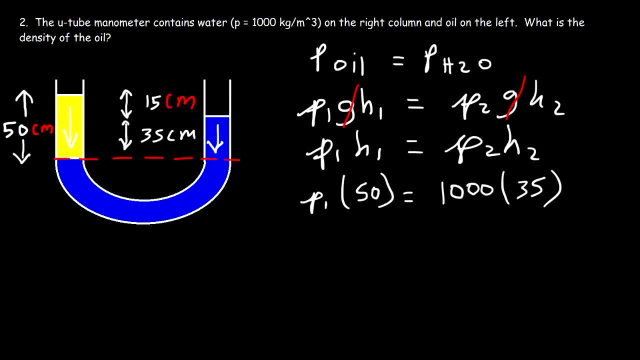 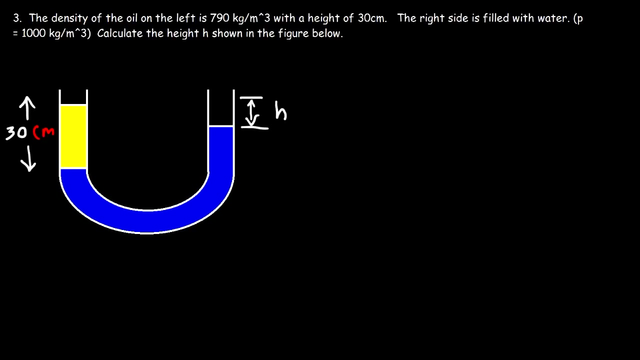 So it's going to be 1000 times 35 divided by 50. So the density of the oil is is 700 kilograms per cubic meter, And so that's the answer in this problem Number 3.. The density of the oil on the left. 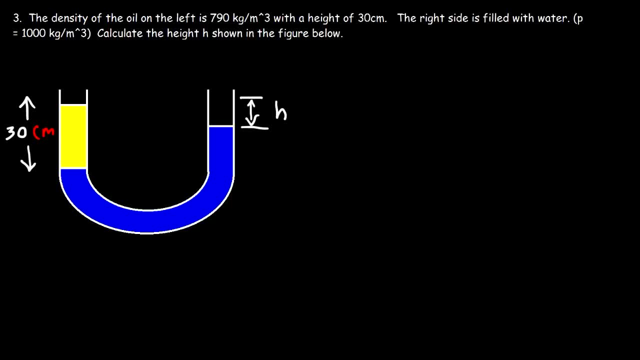 is 790 kilograms per cubic meter with a height of 30 centimeters. The right side is filled with water. Calculate the height h shown in the figure below. So we want to find this value. So go ahead and try this problem. Now let's establish. 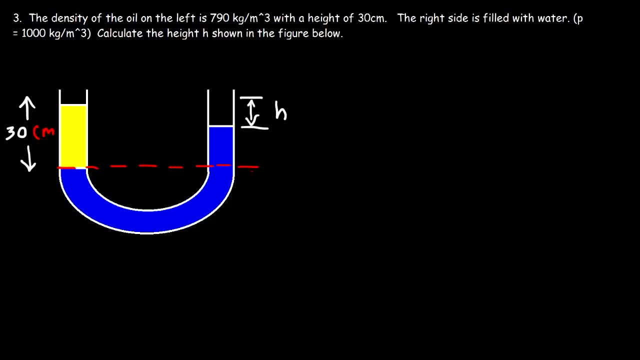 a reference level. So let's call this height h1.. Or rather h2.. That's going to be the height of the water above the reference level. So, just like before, we know the pressure of the oil exerted on the left side. 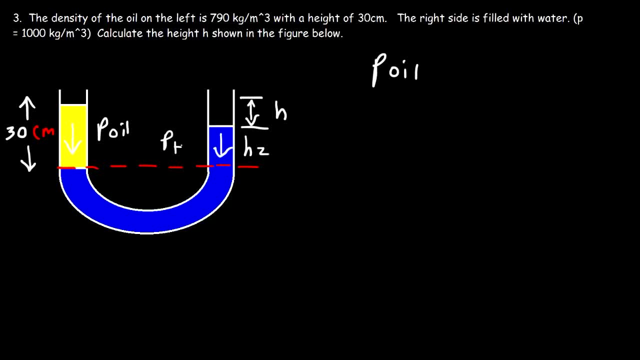 has to equal the pressure of the water exerted on the right side, The portion that's above the reference level, And so that's going to be density times gravity times height. The density of the oil is 790.. And the height of the oil is 30.. 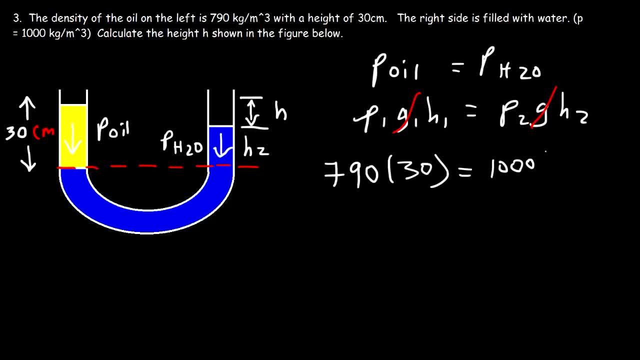 The density of water is 1000.. So let's calculate h2.. So it's 790 times 30, divided by 30.. divided by 1000.. So h2 is 23.7 centimeters. Now we're looking for this h. 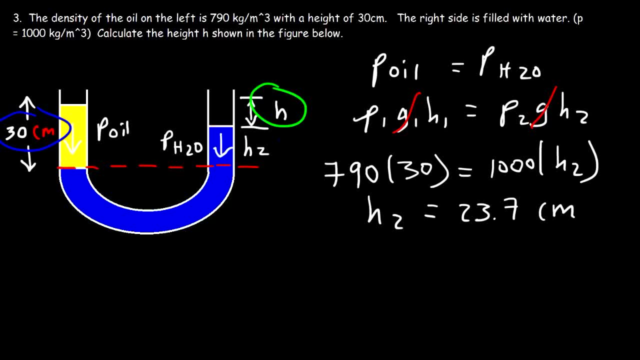 Which is the difference between 30 and h2.. So h is 30 centimeters minus 23.7 centimeters, And so the answer is 6.3 centimeters. So the surface of the oil is 6.3 centimeters. 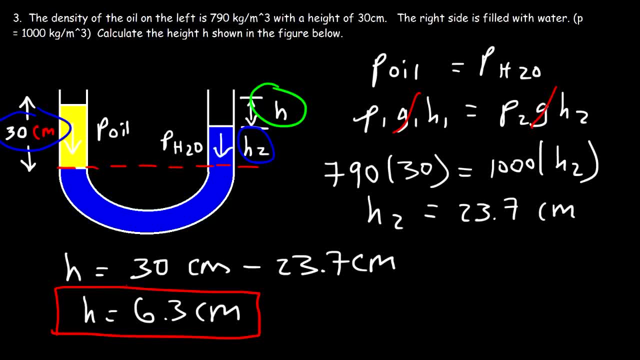 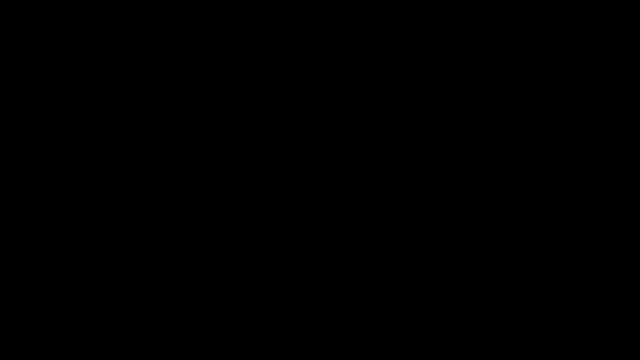 higher than the surface of the water. I'm going to estimate the area of the oil by h2.. Okay, so h is 30 centimeters and h2 is 4 centimeters, And so the difference is that the oil in the oil is 20 centimeters And so